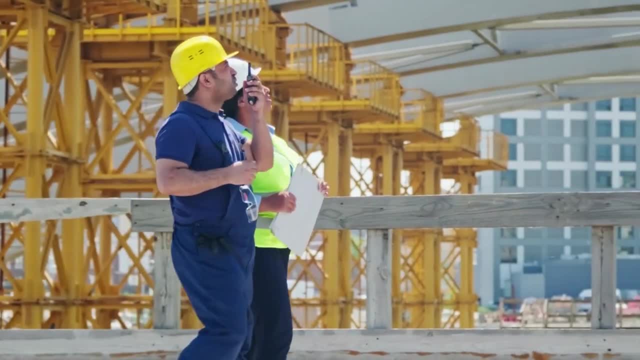 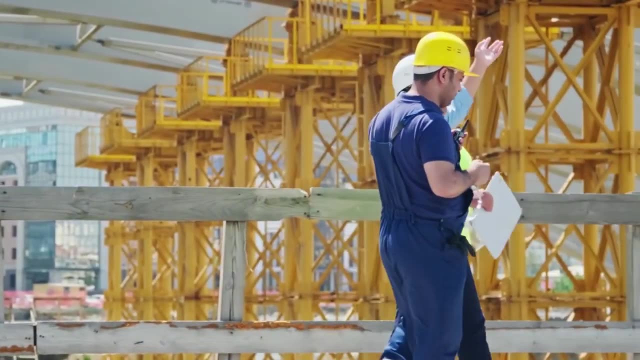 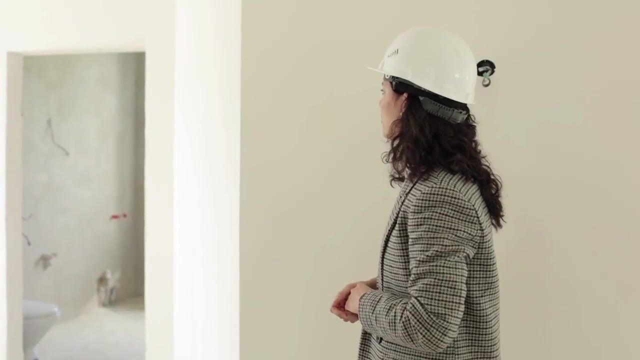 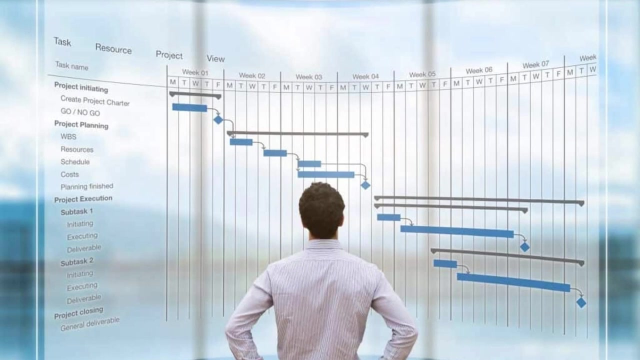 and geologic data. They confirm adherence to construction specifications and safety standards by monitoring project progress, inspecting construction site and verifying calculations and placements. They maintain operations by enforcing project and operational policies and procedures. Civil engineers provide engineering information by answering questions and requests. They also maintain project database by writing computer programs. 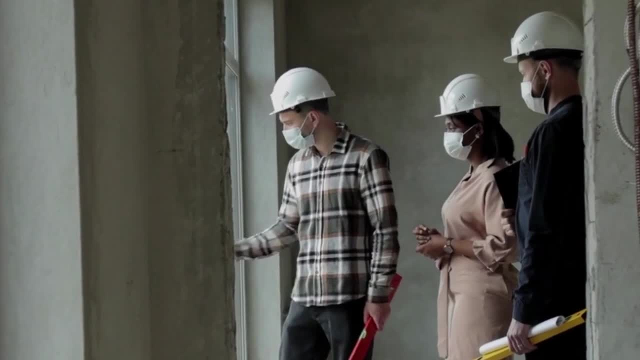 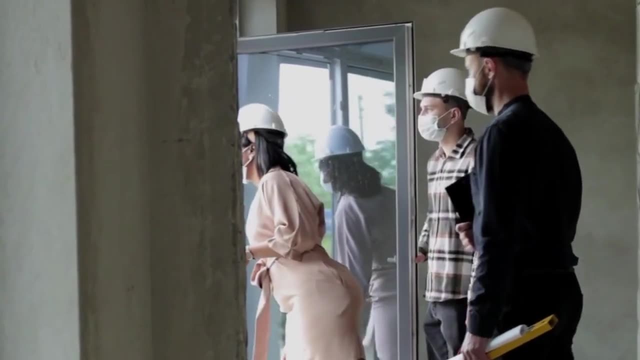 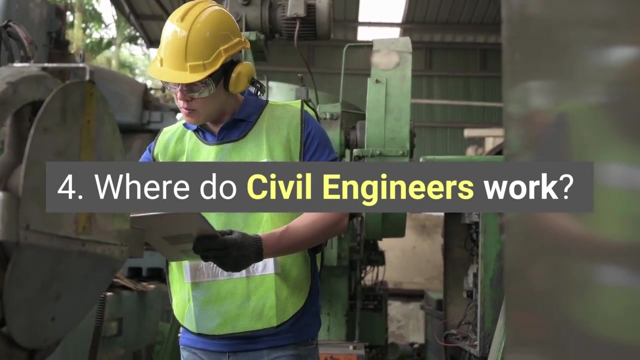 entering data and completing backups. They coordinate with clients and other professional subcontractors and manage project budgets, resources and deadlines. Where do civil engineers normally work? There are several subfields that a civil engineer can build his career. One of the specialization 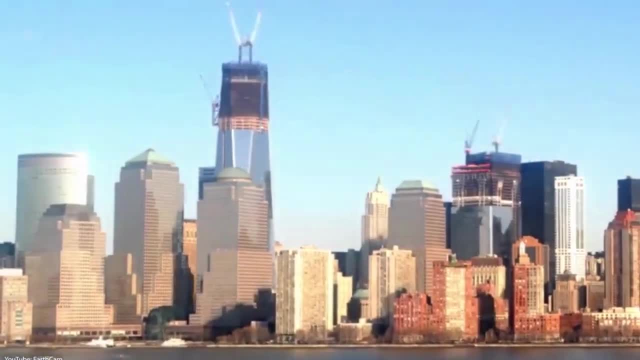 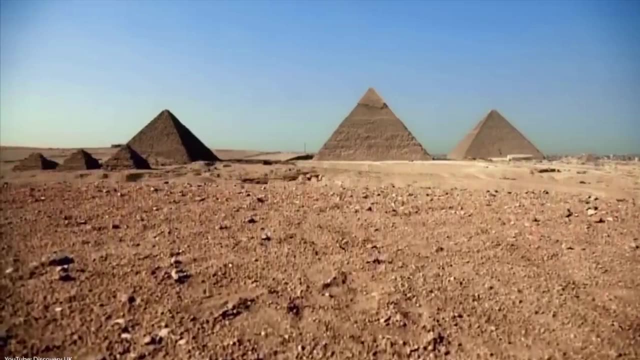 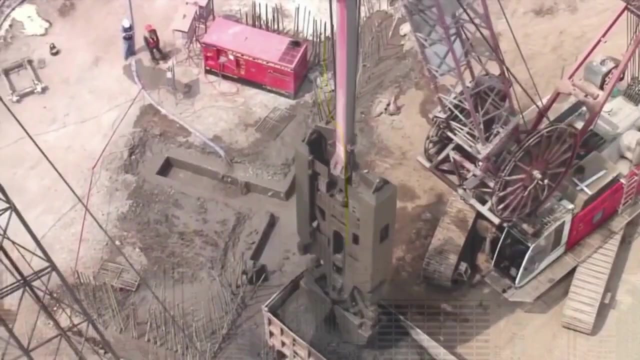 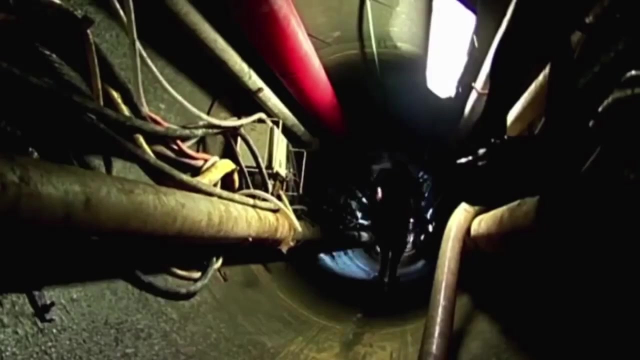 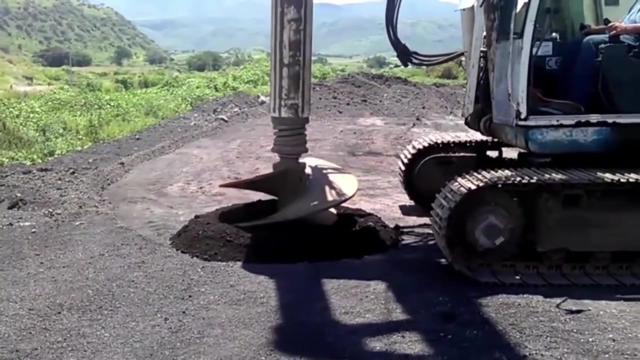 under civil engineering is construction engineering. Construction engineering is involved with planning and execution, transportation of materials and site development. It includes business-like transactions like reviewing contracts, evaluating logistical operations and monitoring projects. Civil engineers are also responsible for the development of building시고 audio of any government or local systems and also promote folks'. 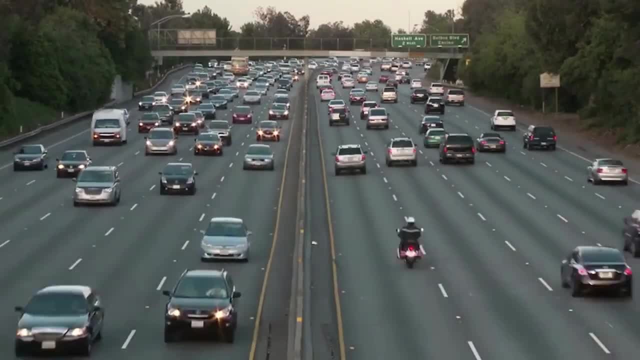 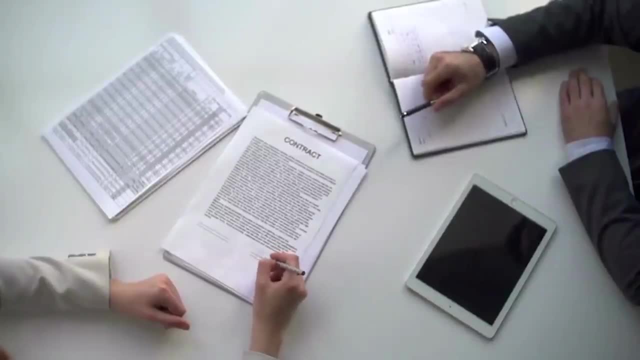 joy to build their offices, hotel and buildings. They also provide environmental tech design systems and CayenneDieU jobs. This kind of technical equipment can provide solutions to conducive to a vibrant community. It involves specifying, designing, constructing and 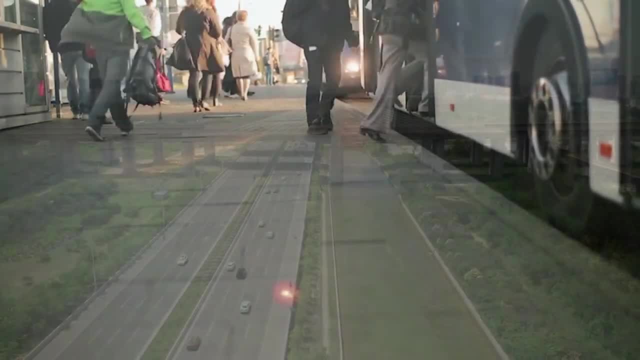 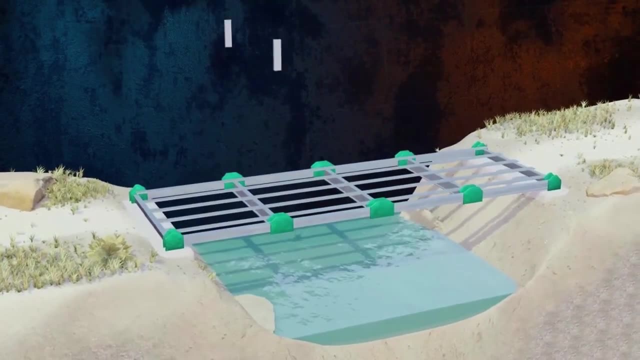 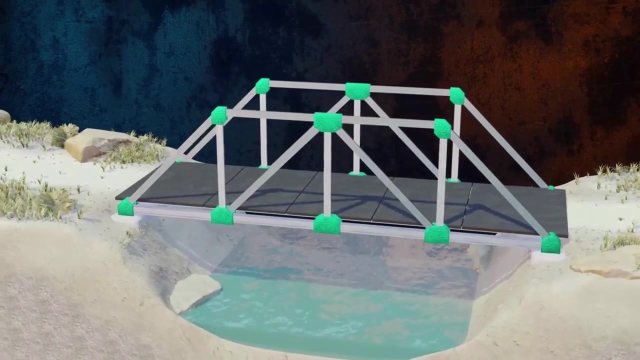 maintaining transportation infrastructure, which includes streets, canals, highways, rail systems, airports, ports and mass transit. Fourth specialization under civil engineering is structural engineering. Structural engineering deals with the structural design and structural analysis of buildings, bridges, towers, flyovers, overpasses, tunnels, offshore structures like oil. 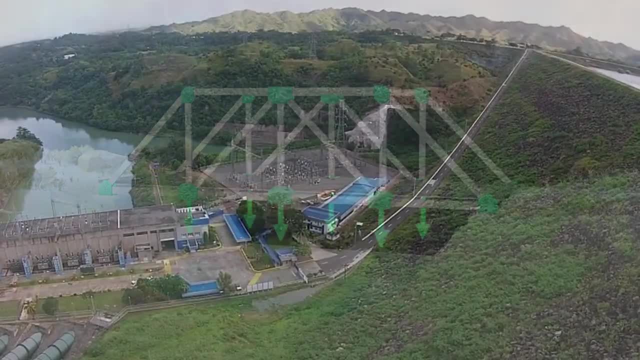 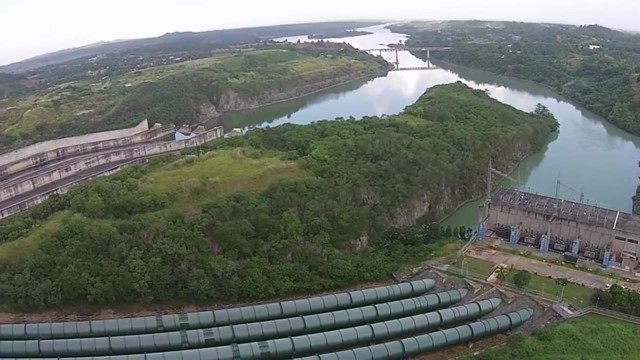 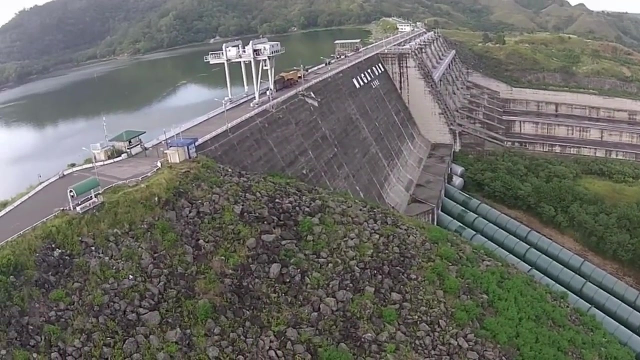 and gas fields in the sea, aerostructure and other structures. Last is water resources engineering. Water resources engineering deals with the collection and management of water as a natural resource. This area of civil engineering relates to the prediction and management of both the quality and the quantity of water in both underground, like aquifers, and 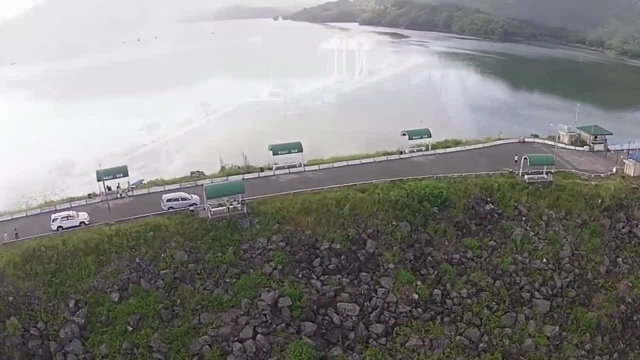 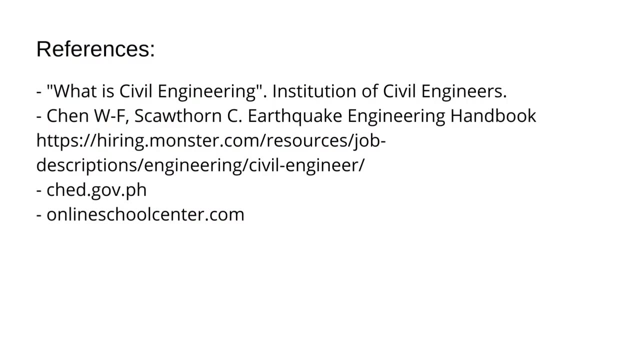 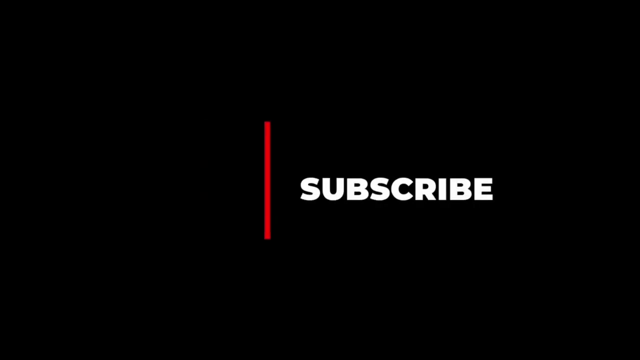 above ground, like lakes, rivers and streams. Thank you very much for watching. See you on our next video, wwwnasagov.